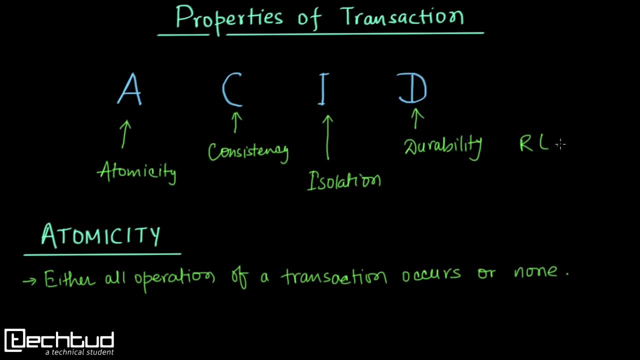 studied to increase the salary. first we need to read salary. so let's say S. then we update salary S equal to S plus 0.1 S and then write S, right? So this transaction contains all those okay, which is there to increase the salary by 10 percent. we have three operations right, so these? 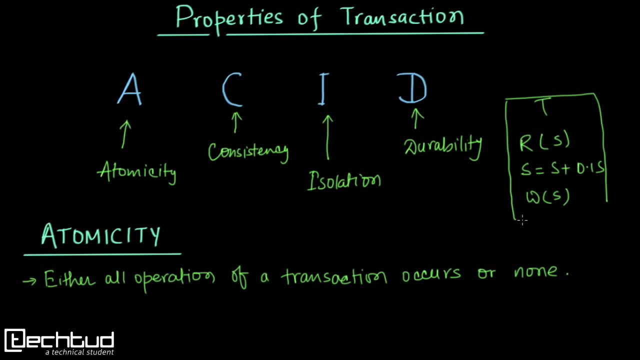 three operations. either all three operations should be completed, all of three, or else none of the operation will will be performed. so there should not be a case when, after this operation, transaction aborts and this is not performed at all. okay, so this cannot be and this is not at all. 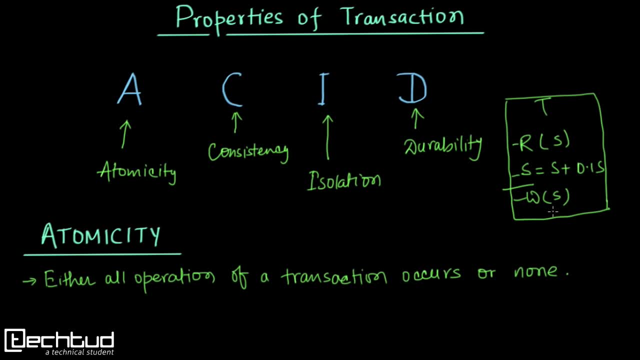 acceptable. okay, this is a basic property that the transaction should be atomic. this property, this atomicity, is maintained by transaction management component of the dbms. okay, so for each property we have someone responsible. we should have someone responsible who will be maintaining or will be ensuring this property right. so for this atomicity, we have transaction. 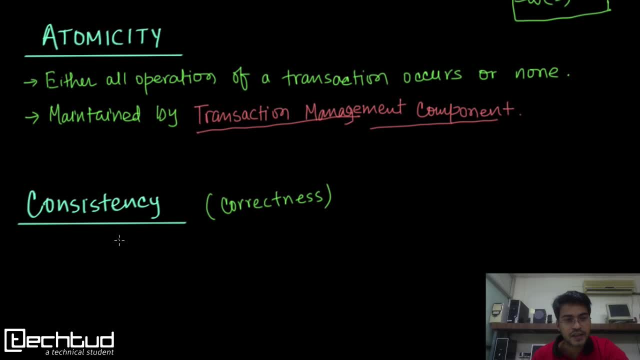 management component: okay. next property is consistency, so consistency refers to correctness. okay, so any transaction should lead to database system from one correct state to, or one consistent state to, another consistent state. a simple example of consistency can be: a value of a is stored and in the same database, a value which is derived from is stored. okay, so let's say this is age, this. 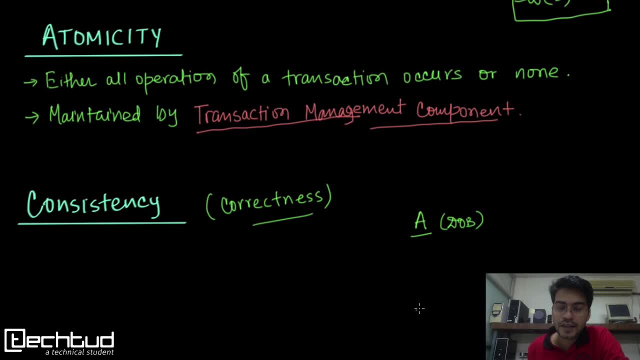 is date of birth, okay. and in the same database we have age: okay, age of the user, fine. so this age is basically derived from this date of birth, right? so now, when we update this or a transaction performs some operation over this date of birth or this value of A, okay, it has to take care of this age. okay. so after this, 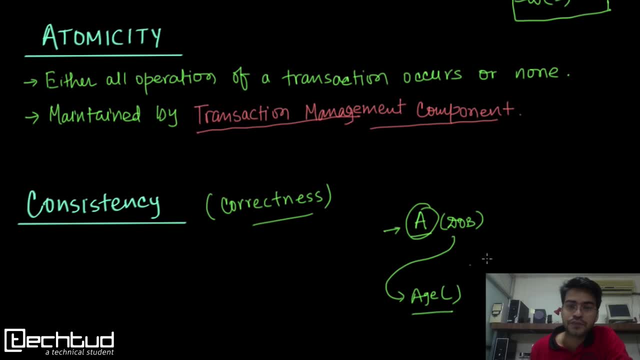 transaction. there should not be a conflict between these two. or in simple word, let's say: I am storing A at two places, okay, A1 and A2, let's say so. transaction has to take care that these two has to be same, okay. so after the, after the transaction is performed, it has to be made sure that value at both 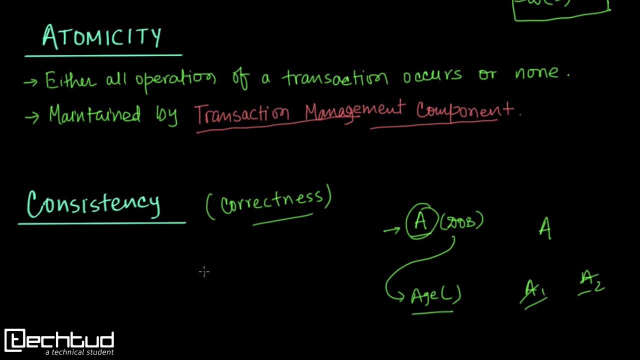 the places has been modified. another example can be that let's say we have two accounts, A and B. we have a balance of thousand rupees here and two thousand rupees here. okay, now some transaction. this one A and this one, let's say, A2. okay, so two different accounts we have. 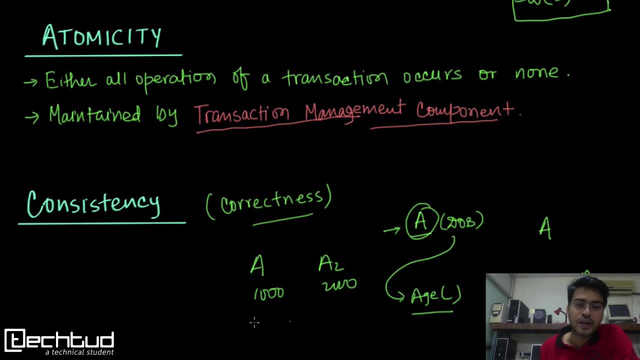 balanced thousand and two thousand, so total balance is three thousand. now if some transaction is made over it, okay. so let's say I am transferring some account from here to here- 50, okay. so this transaction has to be performed in in a correct manner so that after the completion of the transaction, after 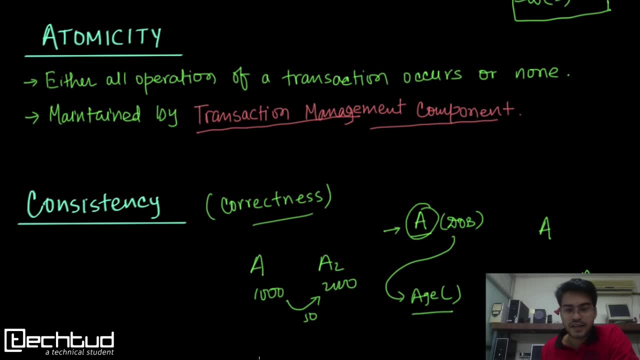 completion of the transaction. final amount should be consistent. that is, here it has to be nine hundred fifty and here it has to be 2050. okay, so the addition of both the balances has to be consistent, consistent, right. so this consistency, you can remember, or you should know that in 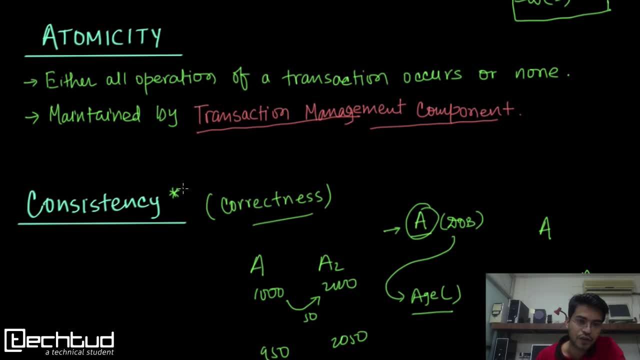 modern databases, this consistency has been compromised. okay, so if you use Facebook, you can see that at some places, number of likes for your page is different, where, at some places, it is showing different. I'll show you quickly, show you an example here. so let's say so this: 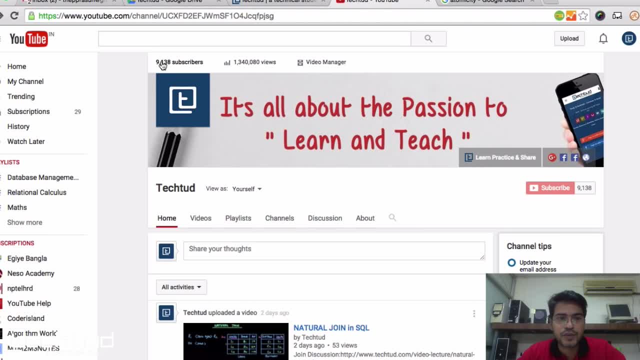 is my youtube channel where you watch these videos and we have here right now, here it is showing, let's say I'll refresh the page, so so you can see that I have 9200 to subscriber on this channel right now. let's go to the subscriber page. so once I click, 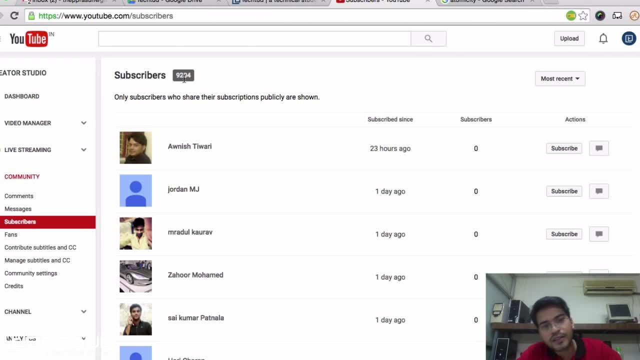 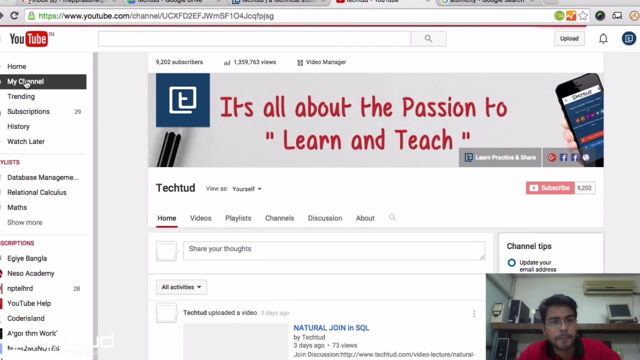 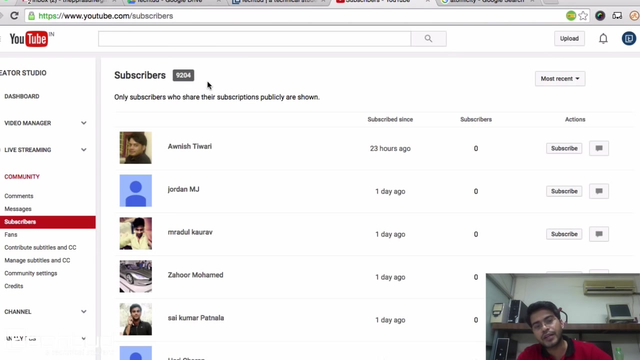 and I go to subscriber page. you can see that here the subscribers are shown as 9200 for right. so earlier it was on the previous page it is 9200. know its old value, it is 9200 to write, but at this page it it is 9200 for right. so you can. 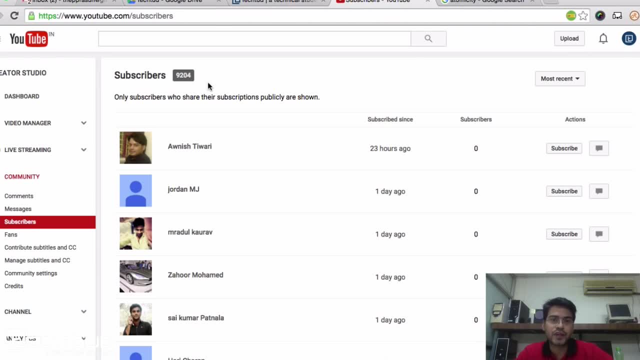 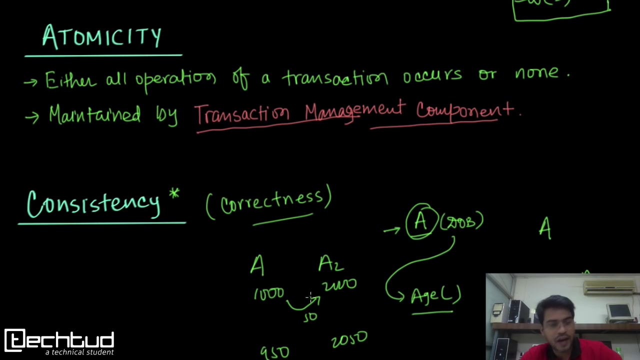 see a clear-cut example of consistency. right, so in modern days, databases, the consistency is compromised just to serve you the data as fast as possible. okay, so this part has been compromised so that the database or this performance of the system is very fast. but in our course, what we have study, we have to. 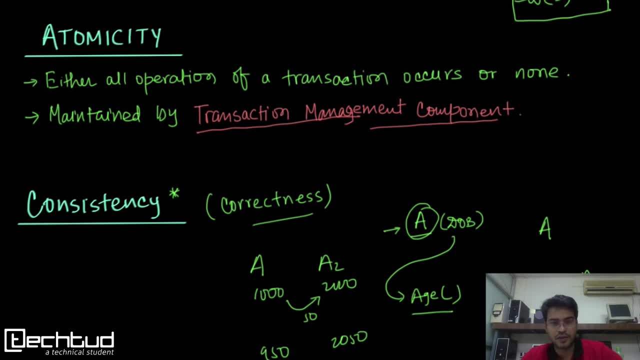 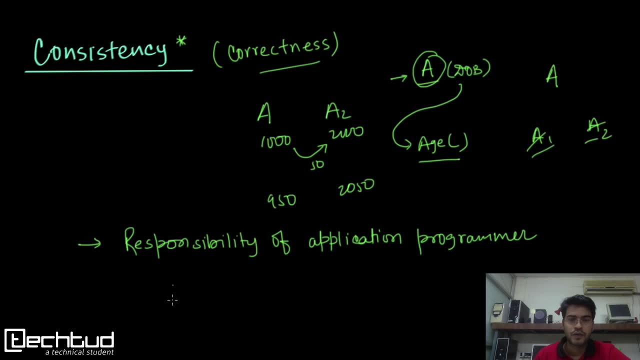 study. we have to consider that it has to be consistent, okay, the value has to be consistent, okay, and each transaction should produce a consistent state. so ensuring consistency is responsibility of application programmer, okay, the one who is programming or creating application over database management system. he has to ensure the consistency of the system. next is isolation property. so isolation. 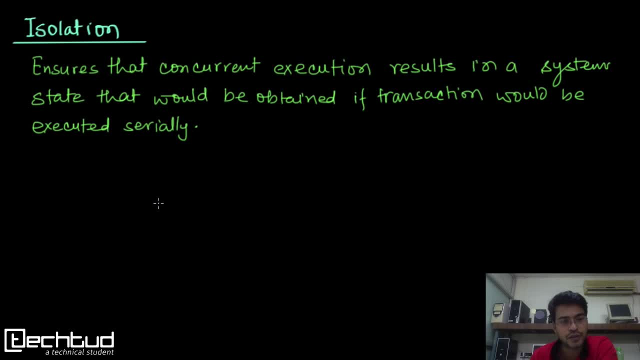 property ensures that concurrent execution. let's say we have transaction t1 and t2 executing ok, so it has multiple operations and it is executing right. so it ensures that the concurrent execution of transaction t1 and t2- t2 results in a system state that would be obtained if transaction would be executed serially- okay. 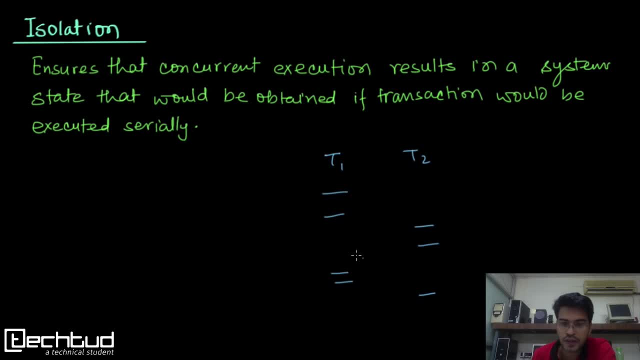 so what i mean to say is: here the transactions are executing concurrently, right, few operations here, then this operation, then this, then this, again right, so it is executing concurrently in interleaved manner. of course. now this execution should result same as if this transaction t1, would have executed completely first and then this t2- right, so this result. 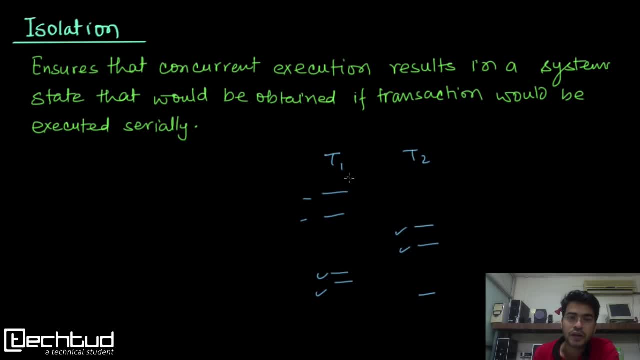 should not be affected if we are executing multiple transactions together. okay, so this is the purpose of this property: isolation- right now. this is the purpose of this property: isolation- right now. this is the purpose of this property. this isolation is managed by concurrency control manager. okay, so it is insured by. 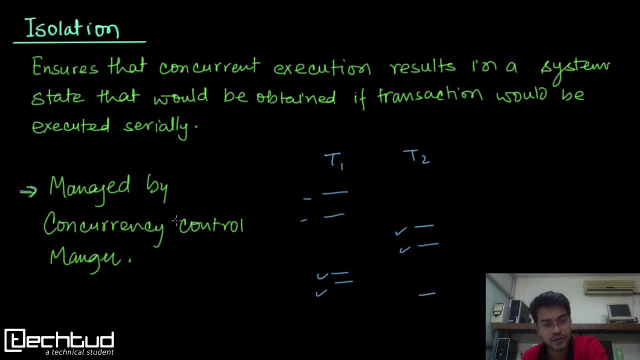 so this is insured by concurrency control manager? okay, and we will study this whole thing in separate lectures. so that is concurrency control, where we will understand how the schedules can be serializable or not, all these things. so we will study all these things, okay, and what can. 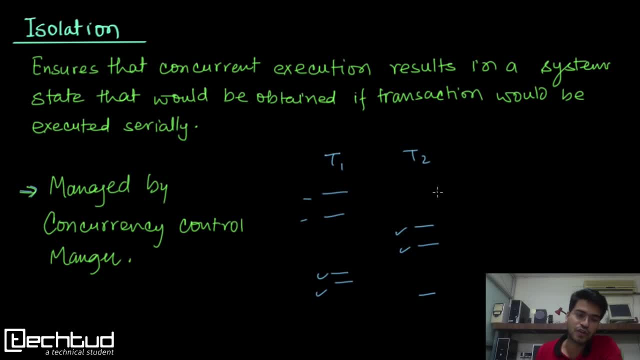 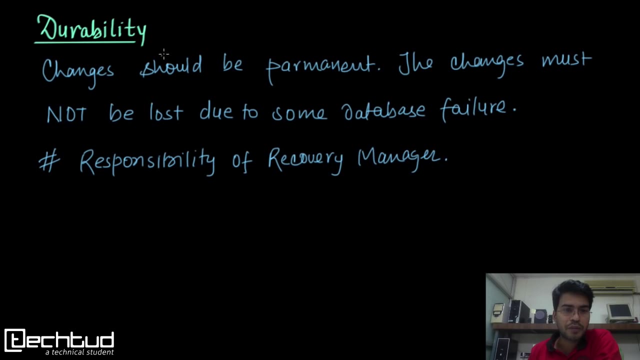 be an equivalent serial schedule for us, given schedule and all okay. so all these things we will study. so this is the purpose of basically isolation property. so now we understand what is isolation, okay. the next property is durability. this property says that changes should be permanent. okay, so whatever changes had been made by a transaction after completion, these 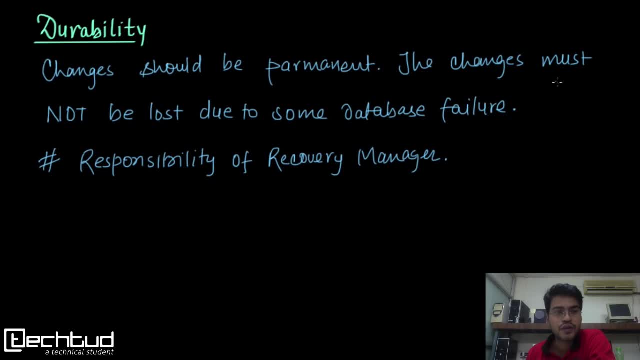 changes should be permanent. okay, these changes should not be lost due to some database failure. okay, so it means that if a transaction is successful, then it should be permanent. okay, so the that all the changes or the effects of transaction should be durable. okay. if a transaction is aborted in between, okay, then we have to roll back, and this is 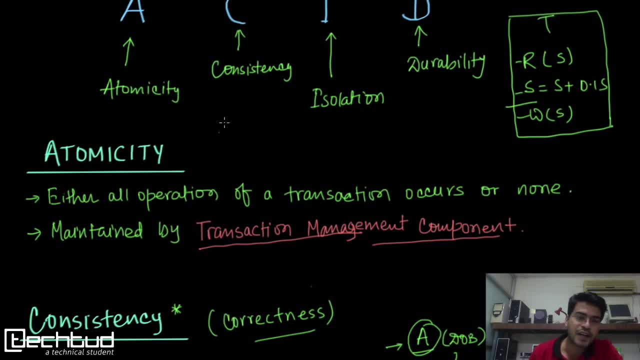 the property of recovery manager. okay, so now we understand the ACID property of transaction, right. so the first one, a, stands for atomicity, okay. so which says that transaction should be atomic? okay, it means that it has to be completed, either completed or it should not occur at all. okay, it means if a transaction 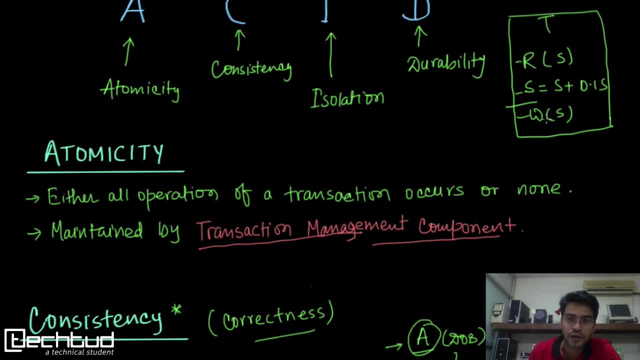 has multiple operations, all the operations will be performed or none. none of the operation will be performed. so if a transaction fails due to some reason here, okay, the transaction has to roll back. okay, it has to roll back to maintain the consistency, and this component is taken care where transaction. 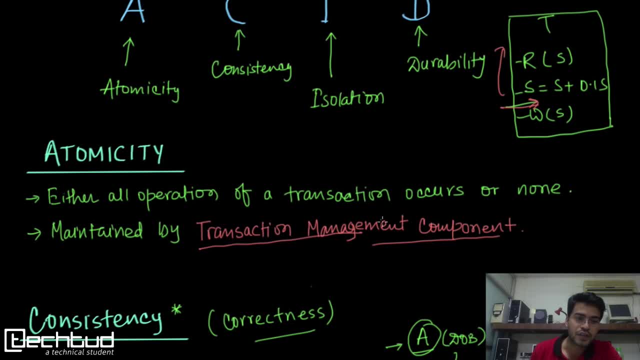 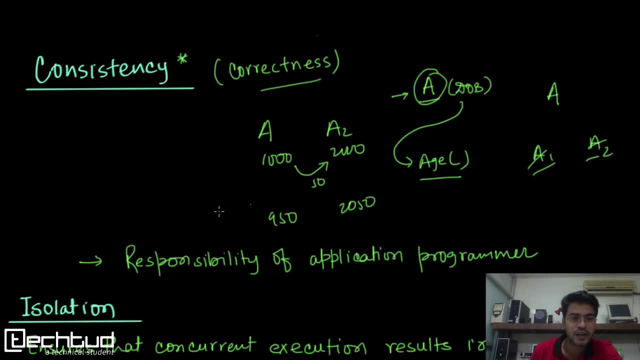 management component. okay now, next one is consistency. it says that the transaction, or any transaction, has to lead a database system to one consistent state, to another consistent state. So the correctness has to be taken care and this is basically the responsibility of application programmer who is programming, who is working on this particular database system. 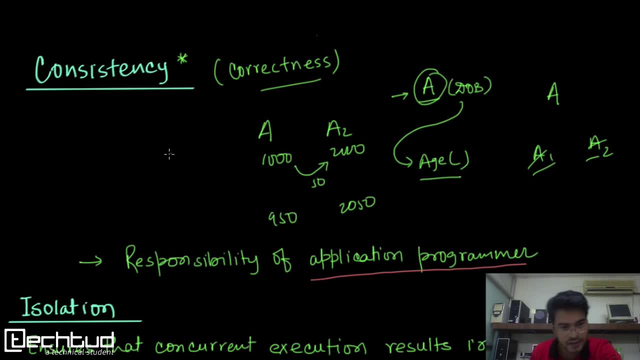 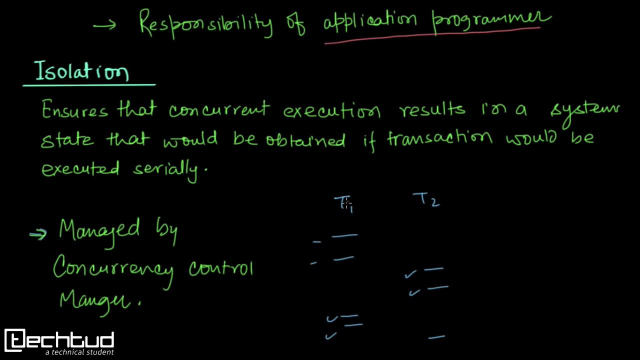 He has to ensure that this system is consistent. Next property: I stands for isolation, So it means that each transaction should act like it is being performed isolatedly. It means that each transaction should be isolated to each other, So, even if they are performing concurrently, the ultimate outcome should be similar to.